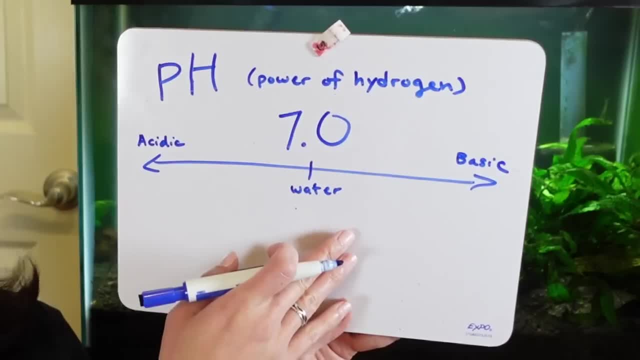 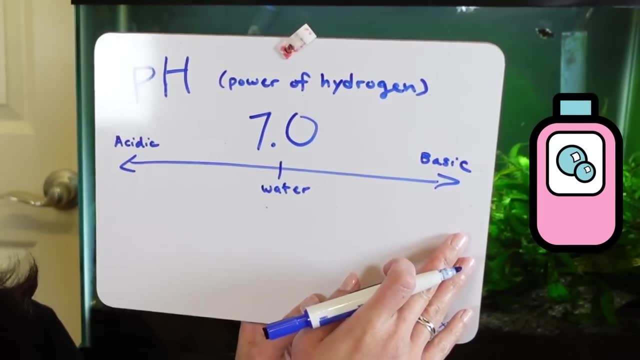 neutral on the scale, which is what pure water is considered. If you are less than 7.0, you're going to have acidic liquids like orange juice, And if you're higher than 7.0, those are basic or alkaline liquids such as soap. 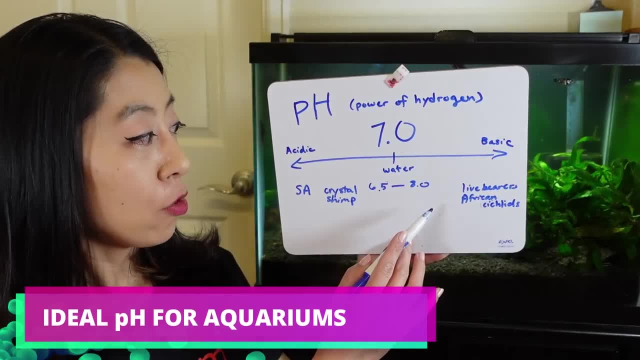 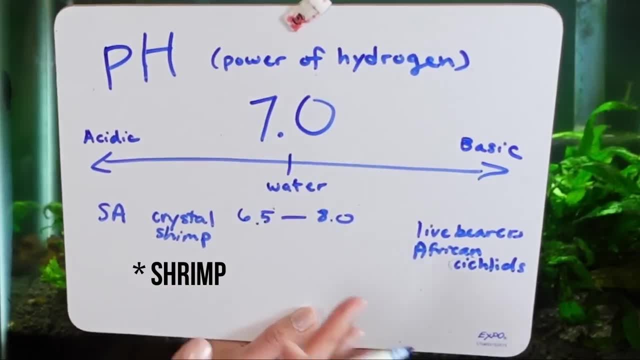 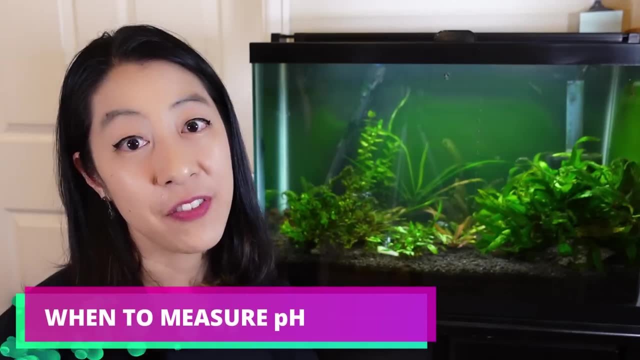 like South American fish, crystal shrimp. they like it on the lower pH side, versus live bears and African cichlids like it on the higher pH side. Hitting a specific pH number usually isn't that important if you're just keeping fish for fun. 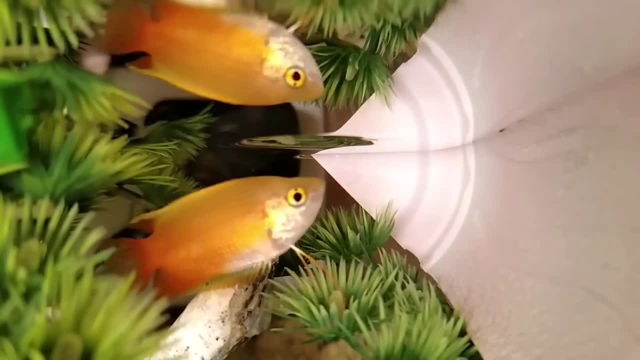 but if you're trying to hit a specific point for breeding purposes or to raise up their fry, that's when you would want to measure pH. or if you see health issues with your fish- 6.5 to 8.0 pH- that's generally fine. However, if you're trying to hit a specific point for breeding purposes or to raise up your fish, 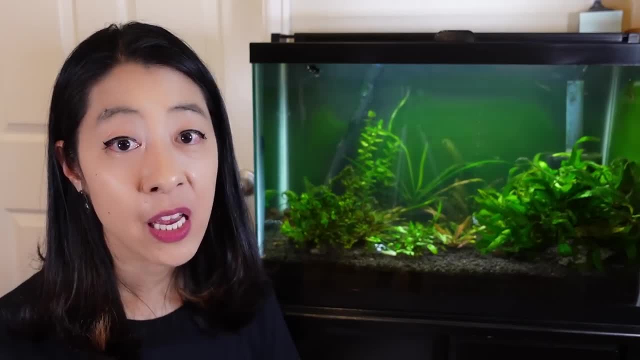 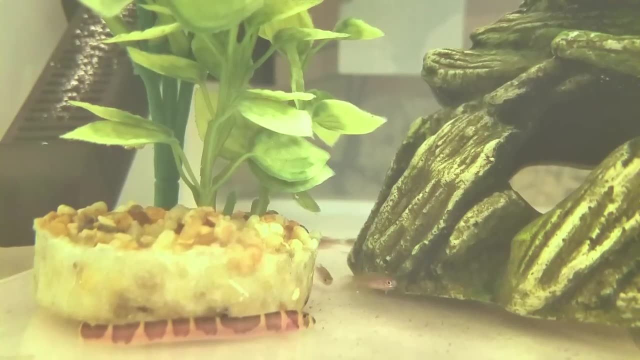 like erratic behavior: swimming frantically, being really lethargic, gasping because the water is burning their gills and their body. all of those are signs that could be caused by the wrong pH. 7.5 to 8.0 pH- that's generally fine. However, if you're trying to hit a specific point for breeding purposes or to raise up your fish, 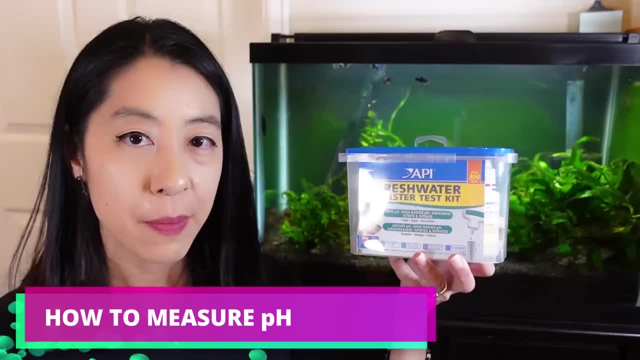 there are different ways that you can measure pH, including well, I've got the API Master Test Kit as well as the Testra 6-in-1 strips. Let me show you how to use them really quickly. 7.5 to 8.0 pH: that's generally fine. However, if you're trying to hit a specific point for breeding purposes or to raise up your fish, 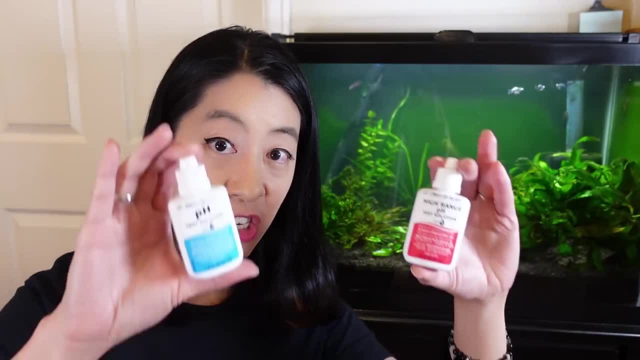 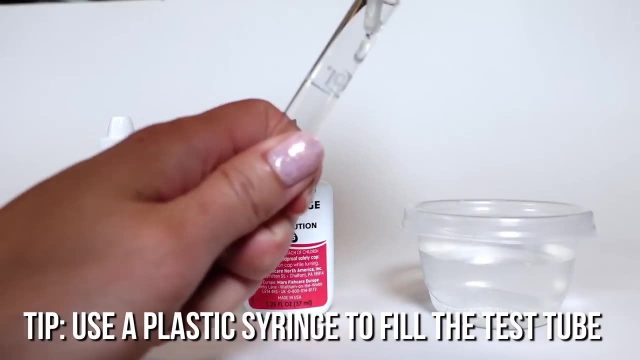 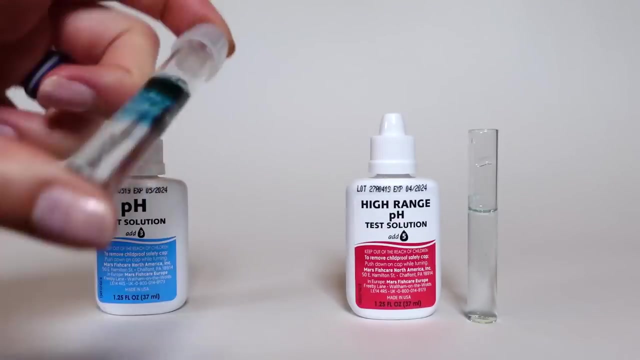 the API Master Test Kit actually comes with two different kinds of pH measurements. One is the regular pH and one is the super high pH. For the regular pH, you're going to put five milliliters of water in your test tube and then add three drops of the pH into the bottle and then invert it several times. 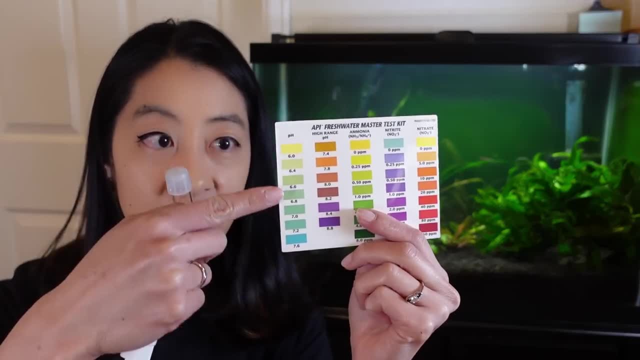 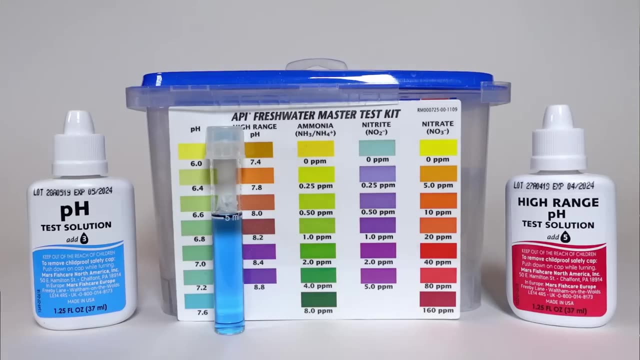 It's going to change colors and then you're going to look at this first chart over here to figure out what the pH is. Now, if the pH is definitely very, very blue, then consider hopping over to the high range. pH 7.5 to 8.0 pH- that's generally fine. However, if you're trying to hit a specific point for breeding purposes or to raise up your fish, 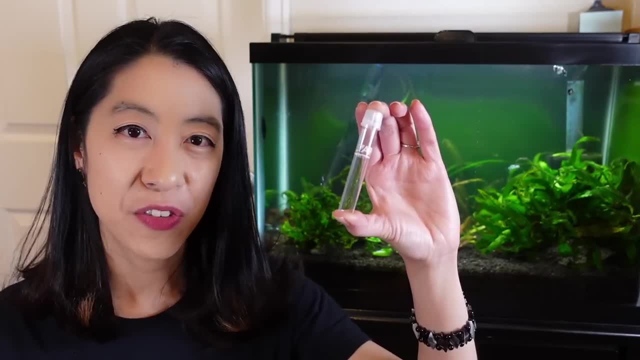 the API Master Test Kit actually comes with two different kinds of pH measurements. Same thing: fill up your test tube with five milliliters of water and then this time use the high pH bottle. You're going to put five drops in the test tube. 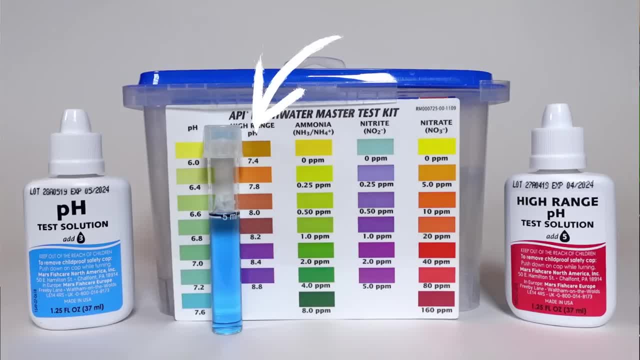 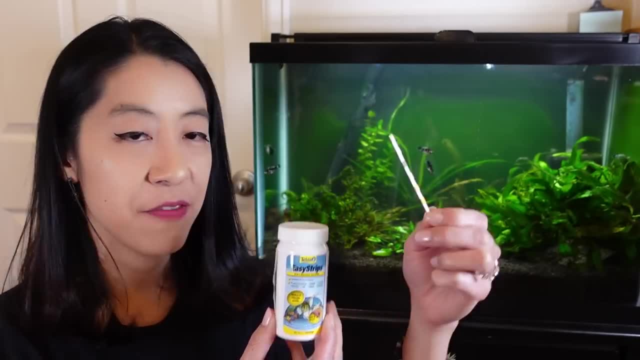 invert it several times, and then this time you're going to use the second column over here to compare the color For the Tetra 6-in-1 strips. it's pretty easy, In fact. I like to cut the strips in half so that you get twice the number to use. 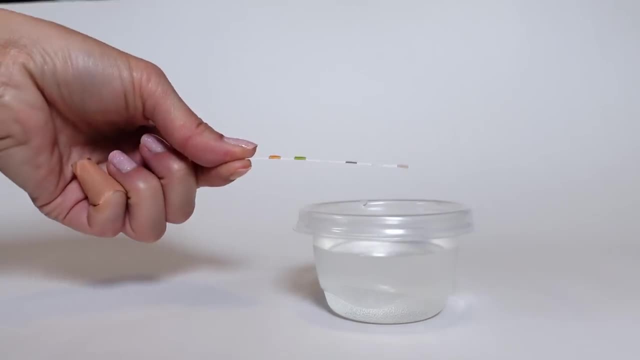 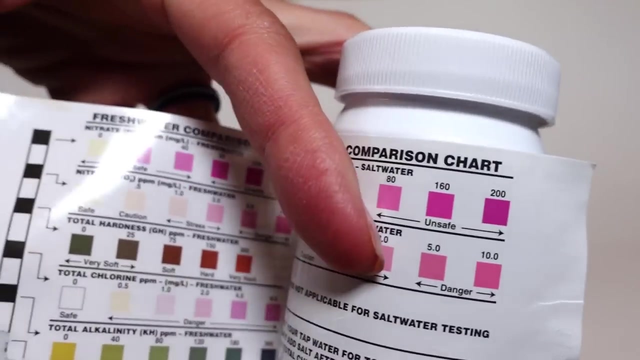 But all you do is dip it in water for one second, take it out and have it flat for 30 to 60 seconds, And then on the back of the jar there's a whole color label system over here so you can help figure out what the pH is. 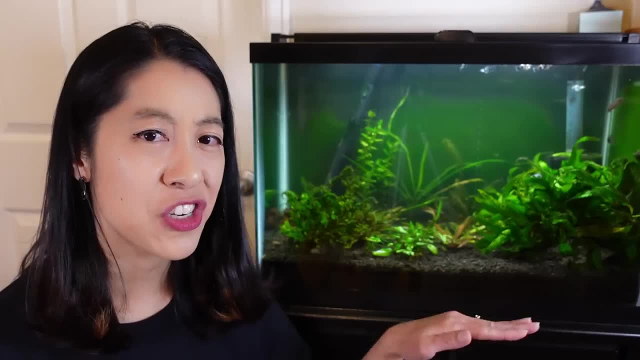 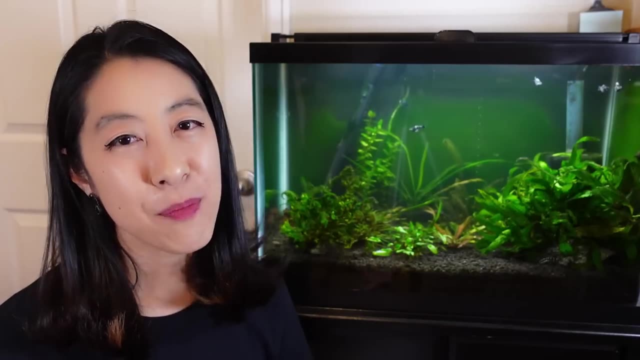 Interestingly, the pH in your aquarium will actually naturally change throughout the day, so the key thing is to maintain a relatively stable pH without any sudden spikes, and most fish will be able to adapt All right. next we're going to talk about KH. 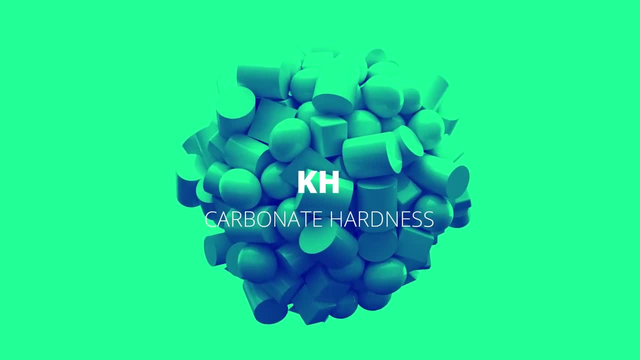 which stands for carbonate hardness, and it measures the number of carbonate and bicarbonate ions in the water. All right, next we're going to talk about KH, which stands for carbonate hardness, and it measures the number of carbonate and bicarbonate ions in the water. 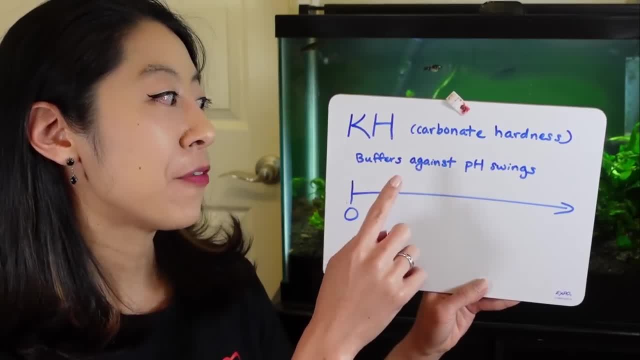 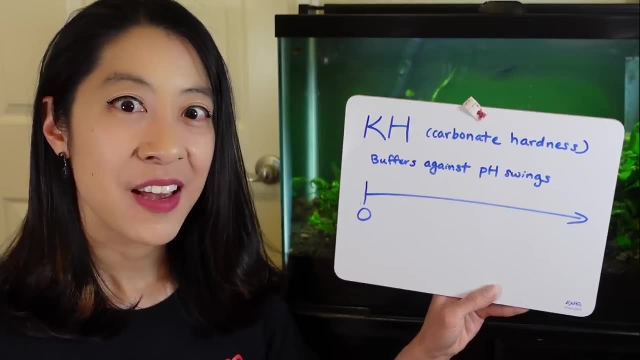 All we care about in the aquarium industry is that it buffers against pH swings, so it helps neutralize acids and prevents pH crashes, which is good, because fish get really stressed out when that happens. So think of it like a trash can, The more KH you have. 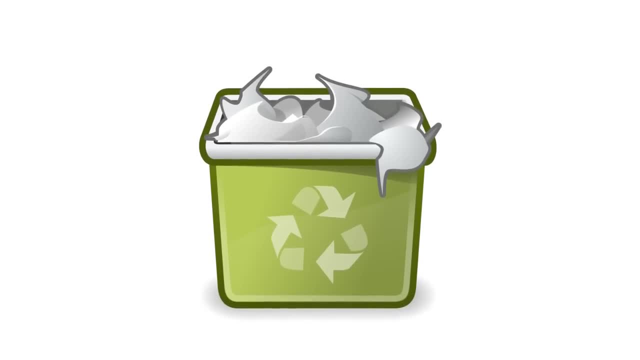 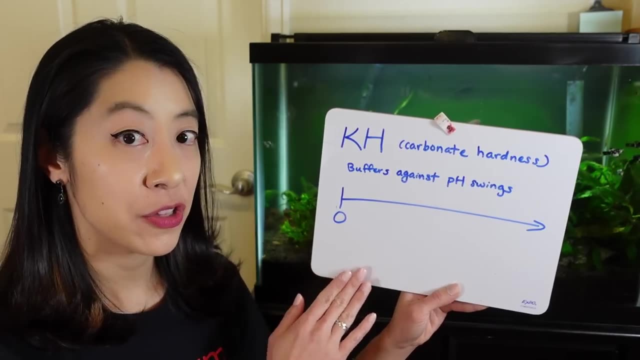 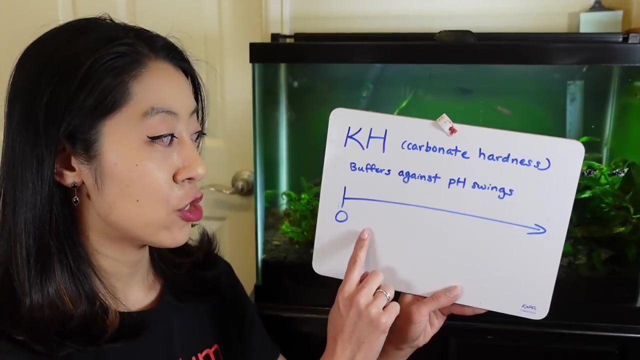 the larger your trash can is, and once that trash can overflows, that's when your pH is going to crash. So a lot of people that have really low KH. they're going to put things like crushed coral and other supplements, which we'll get into in a second, to help increase their KH trash can. 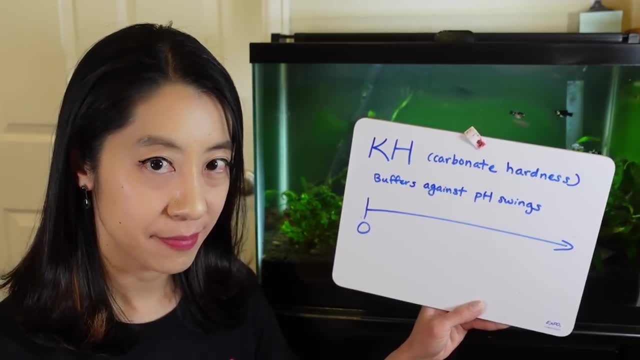 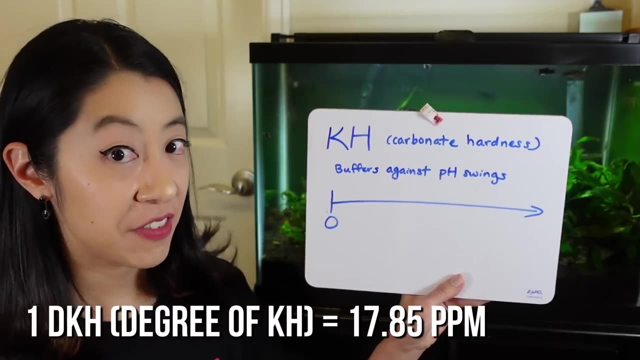 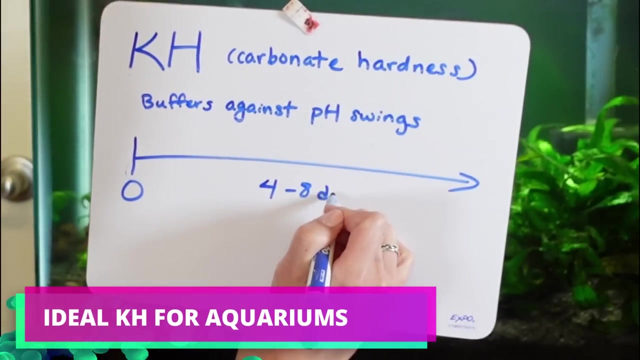 so that that pH won't swing wildly too much. Now KH is measured in degrees as well as parts per million or ppm, so I think one degree equals 17.9 ppm, and the ideal range for a freshwater aquarium is going to be between four to eight degrees of KH, which is about 70 to 140 ppm. 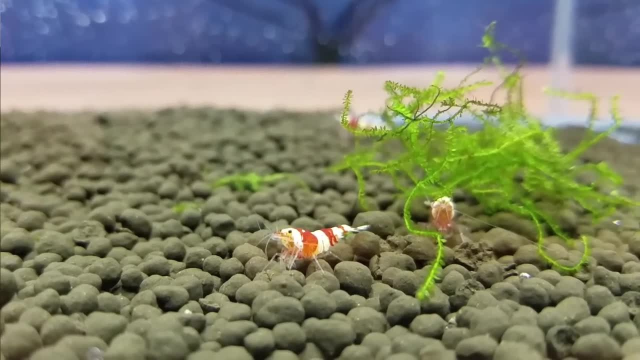 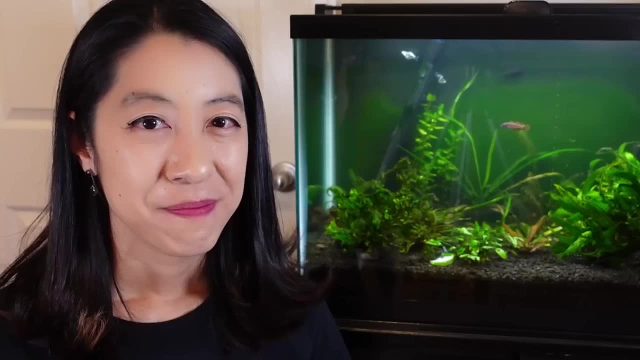 There are animals that have specialized requirements. so if you have discus or crystal shrimp, they like it on the low KH side and then African cichlids definitely like it much higher. The times when you would want to measure KH include, you know, if you want to make sure. 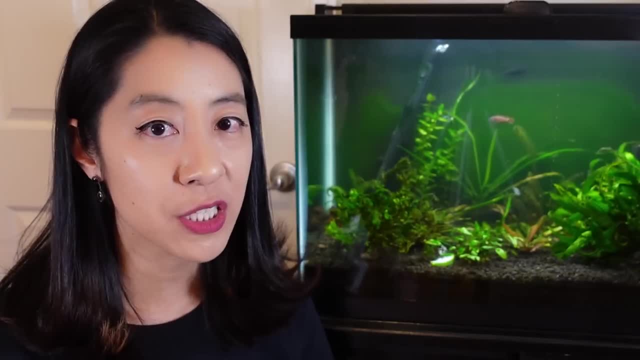 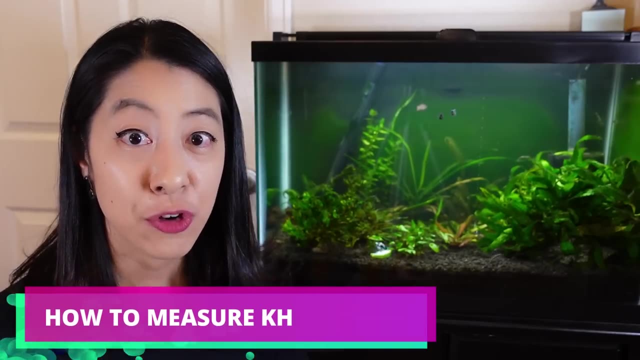 your KH isn't too low, so that it won't cause those pH crashes, or if you are trying to specifically raise or lower it because of a specific animal you're trying to keep. As for measuring KH, you can again use the Tetra test strips that I mentioned before, or API also has a GH. 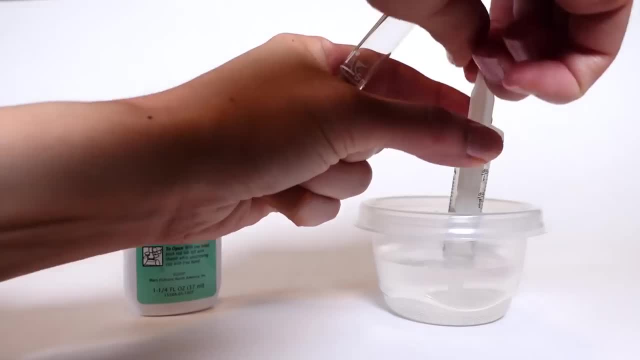 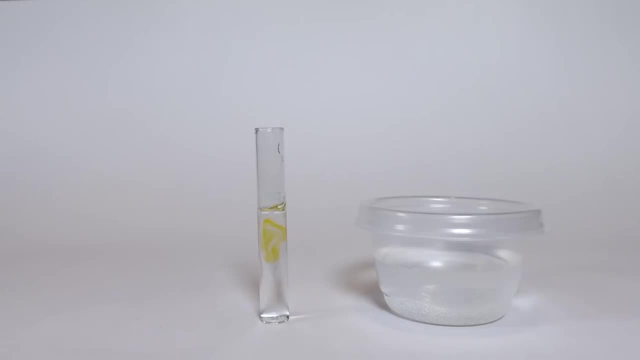 kit which I'm going to quickly show you how to use. So how to use the API KH test is simply fill up your test tube to the five milliliter line. add one drop of the KH in here, invert it a few times. 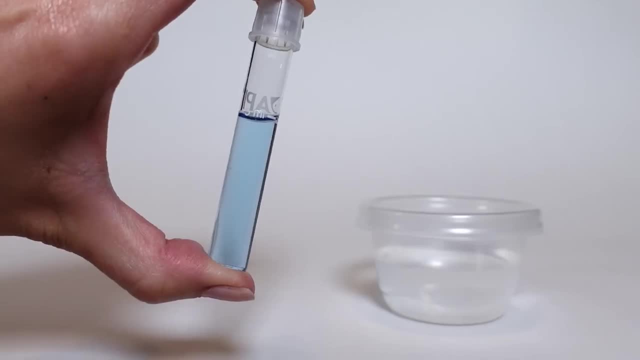 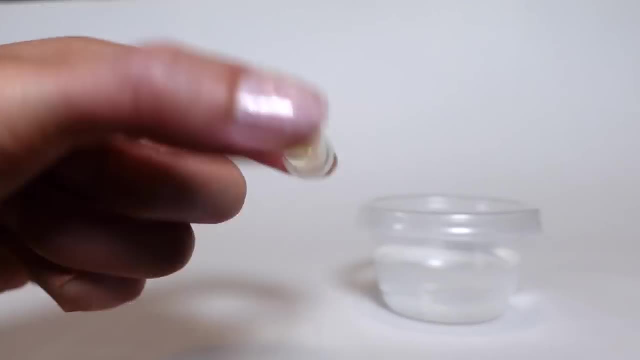 see if it changes color from blue to yellow, If it doesn't add another drop. you want to keep count of how many drops you had to add in here. invert it a few times and when the number of drops finally changes this from blue to yellow, that is the number of dKH, or. 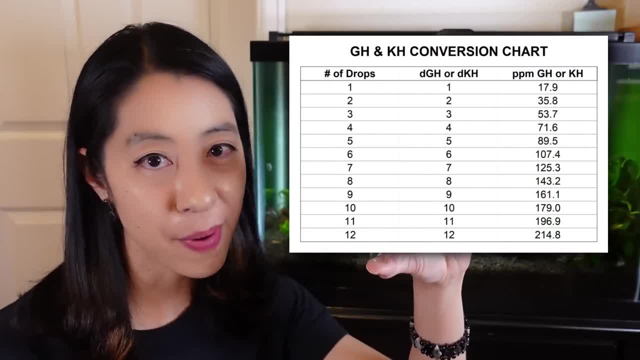 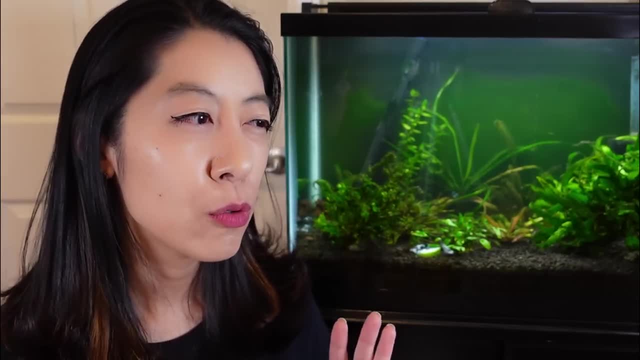 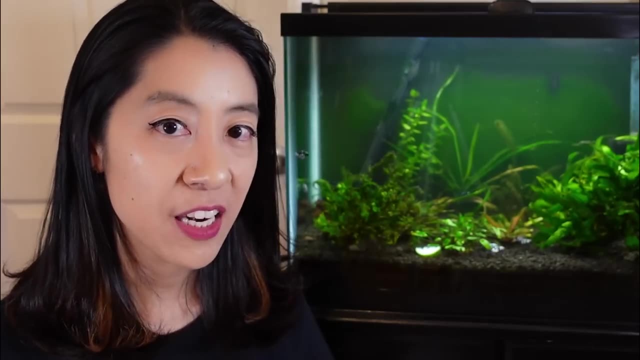 degrees KH that the liquid is, And there's a chart in the back to convert it to ppm as well. In general, most people don't want their KH to be really low, like below two degrees or 36 ppm, So if you're like me, I'm going to include instructions at the end on how to raise that. 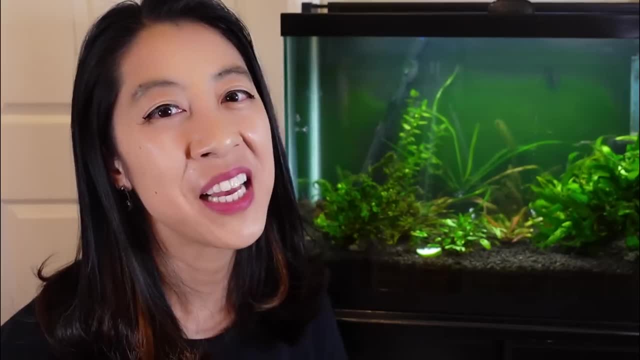 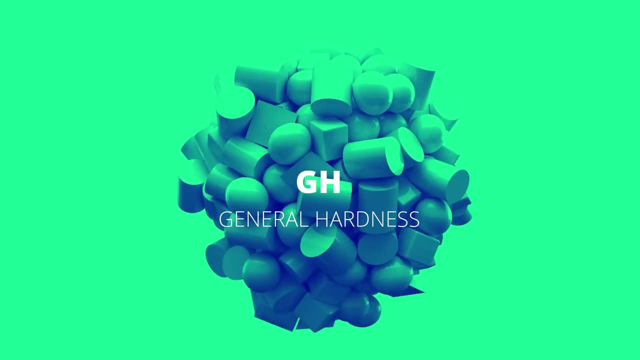 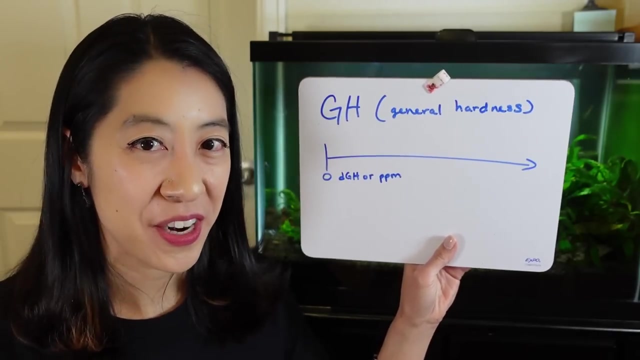 number And again, the exception is if you're trying to specifically raise animals that like low KH. Our last category is GH, or general hardness, and that measures the amount of calcium and magnesium Ions in the water and it basically refers to how hard or soft is the water in your aquarium. 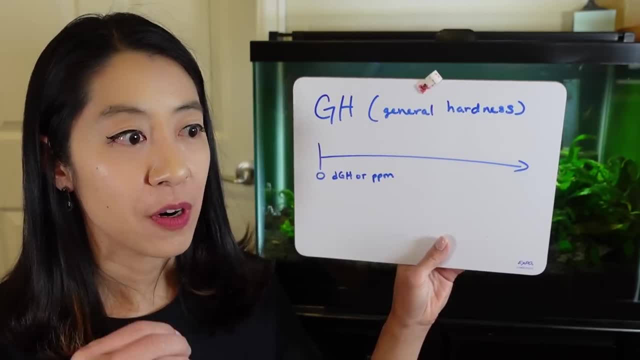 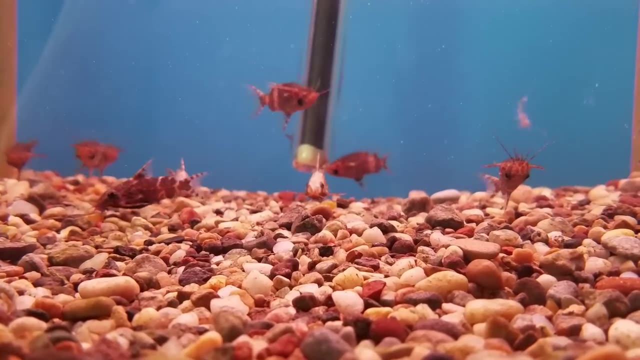 And it's one of the easiest methods we have to measure the number of salts and minerals that are needed for healthy biological functions in your fishes. you know muscle and bone development, the molting of shrimp, snail shell development, as well as plant growth. 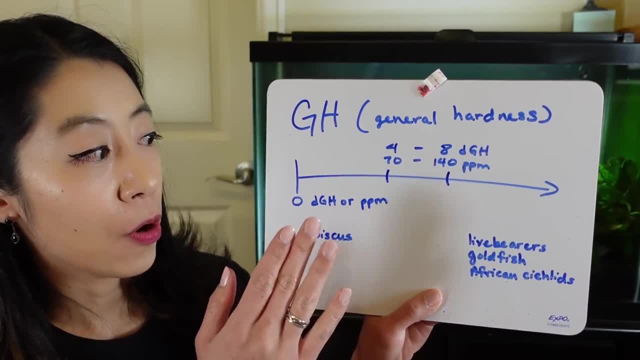 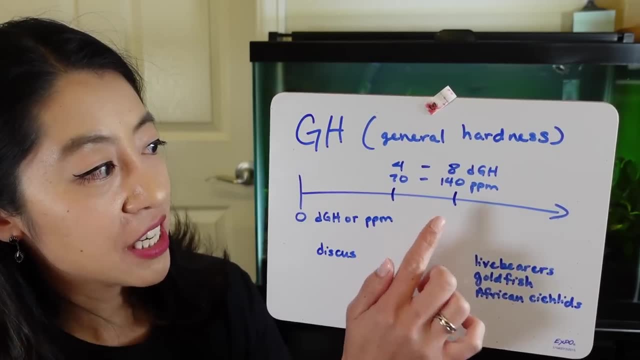 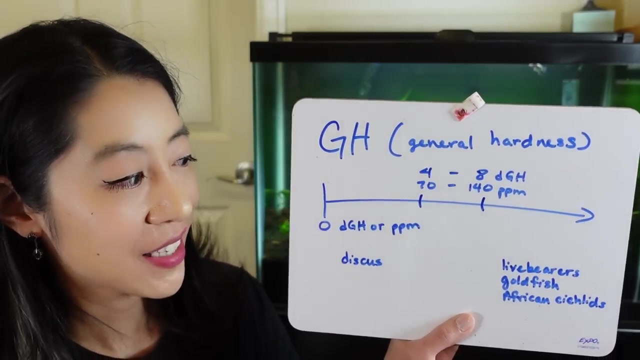 As with KH, GH is also measured in degrees or ppm, And same thing the average freshwater aquarium. it likes to have four to eight degrees, or 70 to 140 ppm. However, there are certain animals that definitely want a lot more minerals in their water, such as live bears, goldfish and African 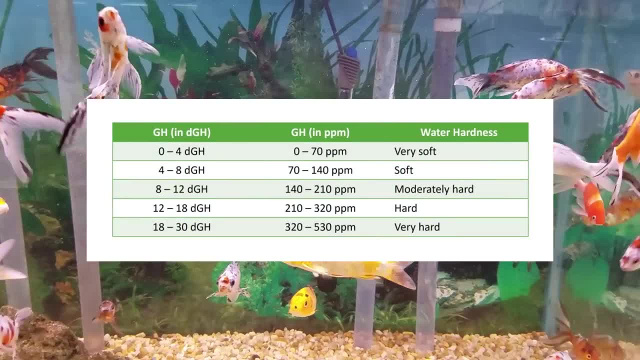 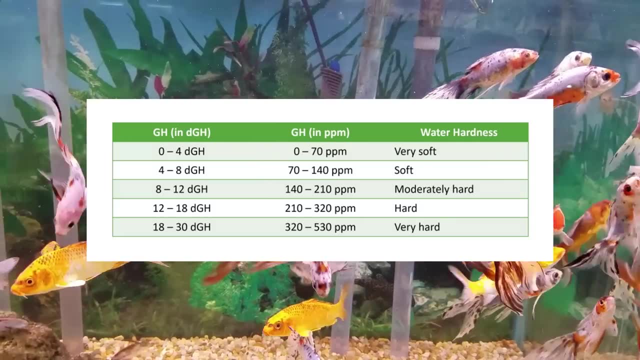 cichlids, And I'm going to include a chart right here that kind of shows you roughly what is considered. you know, soft versus hard water when it comes to degrees of GH. The times you should measure for GH are A if you're obviously trying to measure or reach a. 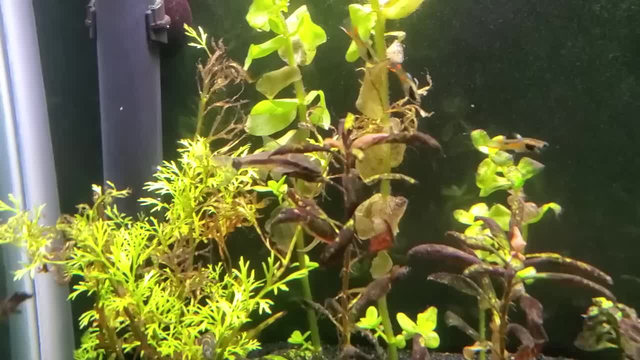 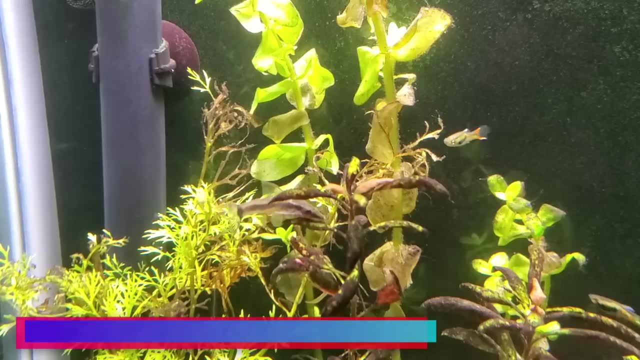 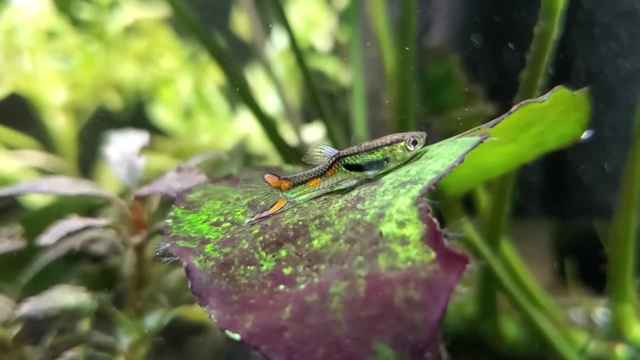 certain level B if you notice health issues. So I mentioned before how my plants were all melting. I'm going to link down in the description below. but we have a whole blog article on how to notice certain types of nutrient deficiencies Your fish. they may have be showing like lethargy, slow growth, faded. colors that kind of thing. Your shrimp may actually die while molting if they don't have enough of these minerals. And then your snails: you may see thin flaking or even holes in their shells. Now remember that GH actually measures both calcium and magnesium ions. So 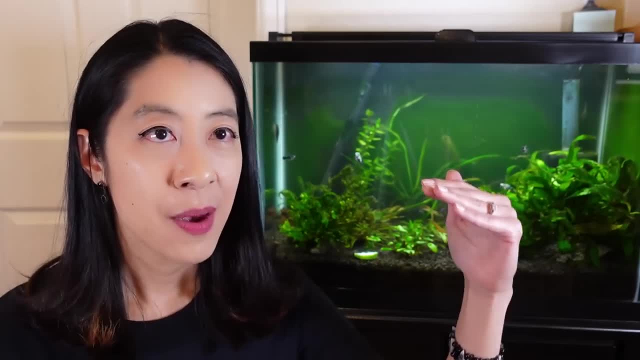 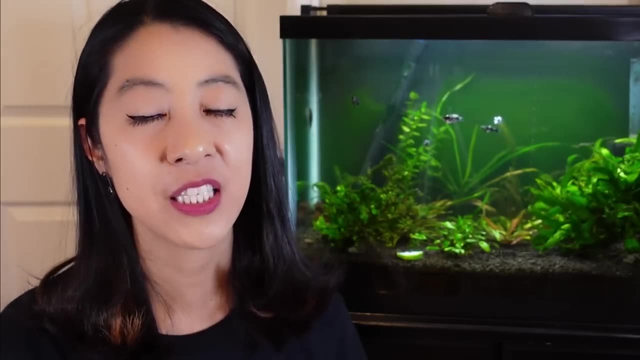 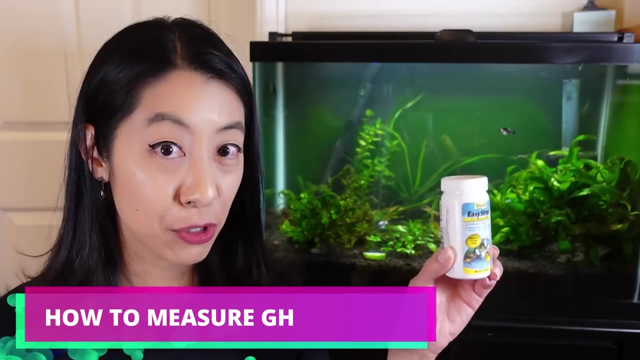 it's possible that you could measure a really high GH, but it turns out it's actually all magnesium ions and you have, like, no calcium. So the only way to get that granularity and measurement is to get a calcium specific test kit to find out what that GH is made of. To measure GH again, you can use 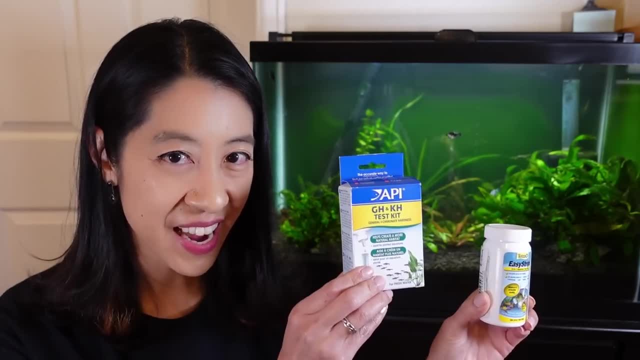 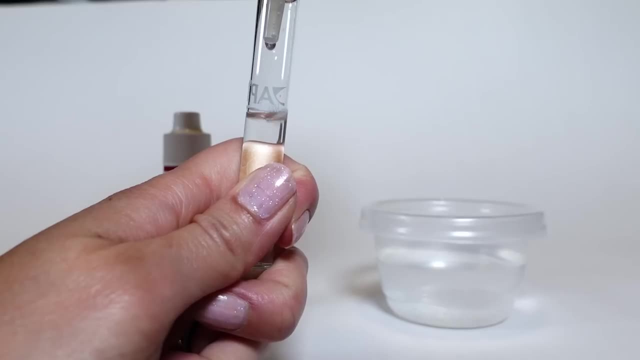 the Tetra six in one strips or get the API GH and KH test. Let me show you how to use this one. It's really similar to the KH test in that you fill up to five milliliters of water. use the GH bottle. 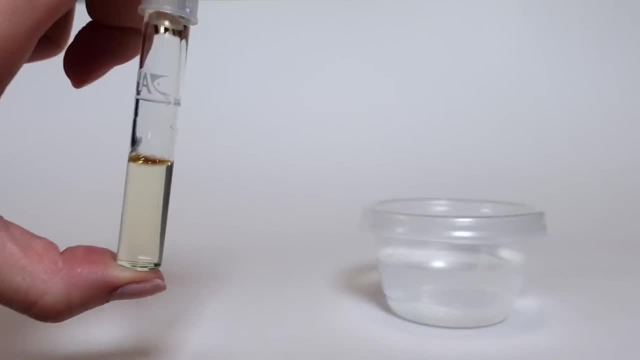 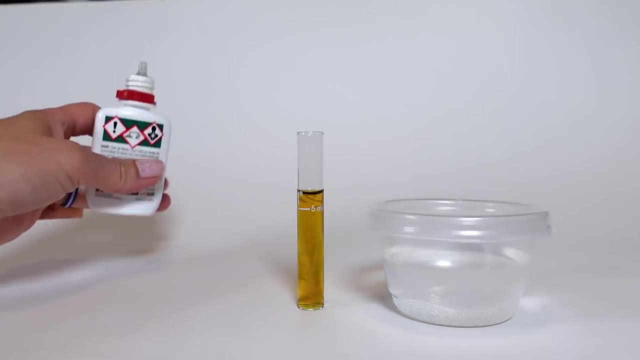 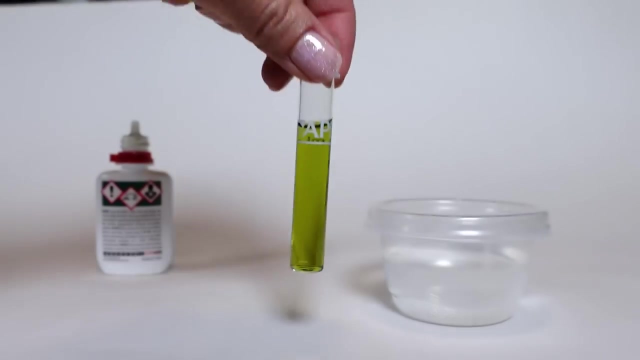 to add one drop, invert, And this time you want to see how many drops it takes to convert the color from orange to green When you've added that last drop of GH and it turns finally to green. that is the degrees of GH that you have And again there's charts in the back to convert it to PPM. 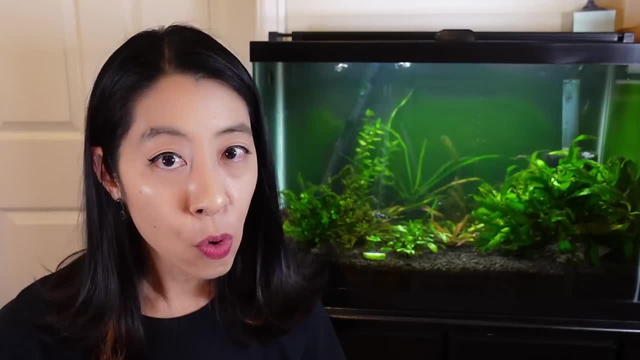 Bottom line. don't let your GH get too low, because then you could see poor health and even death. So you want to make sure that you're measuring the right amount of GH And if you're measuring the right amount of GH, make sure you're measuring your GH and KH, So that way you're 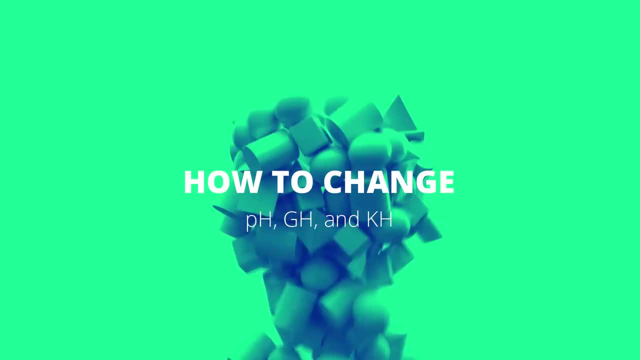 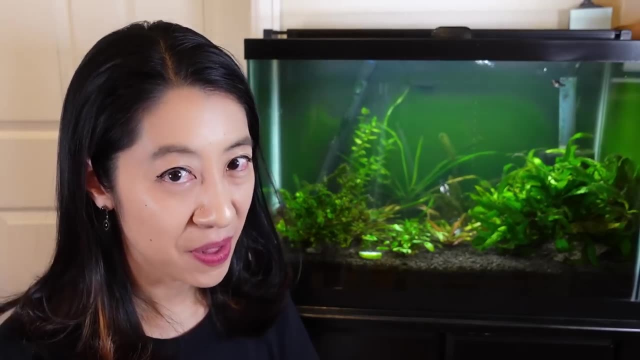 getting the best results And you don't want to lose health and death in your animals and plants. In this last section, I want to teach you how to lower or raise your PH, GH and KH. Now just word of warning: there are many, many methods on how to do that, And some of them are. 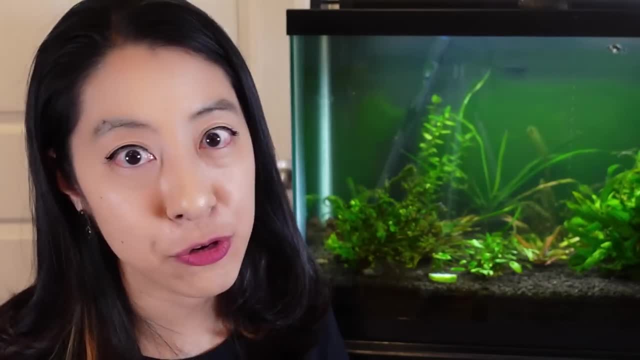 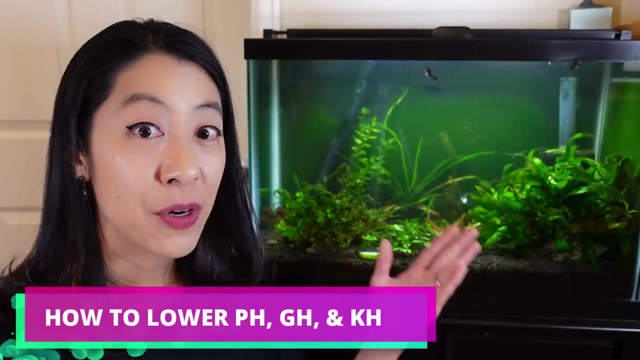 very potent, very effective and very dangerous in my opinion. So I like to err on the side of caution, using much gentler methods. So, for example, in order to lower the PH, GH and KH, one method you could do is just minimal water changes to. 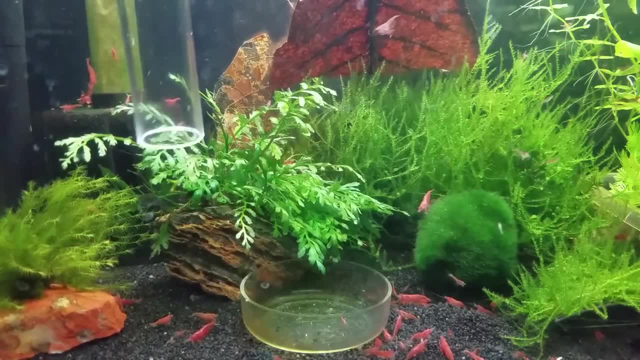 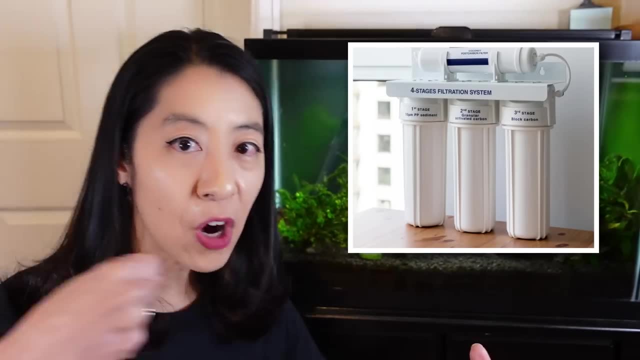 naturally acidify your aquarium over time and lower that pH. Also, you can use an RODI unit- reverse osmosis, deionized water system- to strip all of the minerals out of the water And then, if you need, to add back in a certain amount.